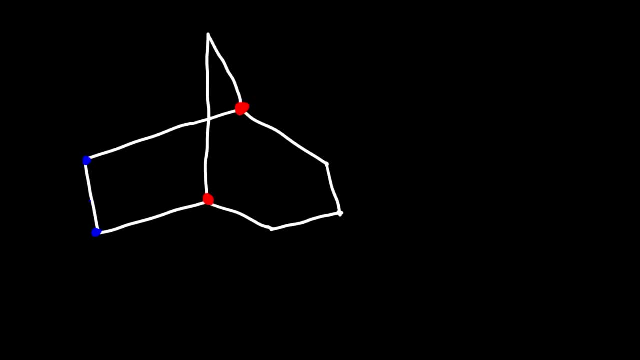 left side, we're going to pass through two carbon atoms. On the right side, we're going to pass through three carbon atoms and at the top there's one between the two bridgehead carbons. So to name this compound, it's going to be bicyclo and 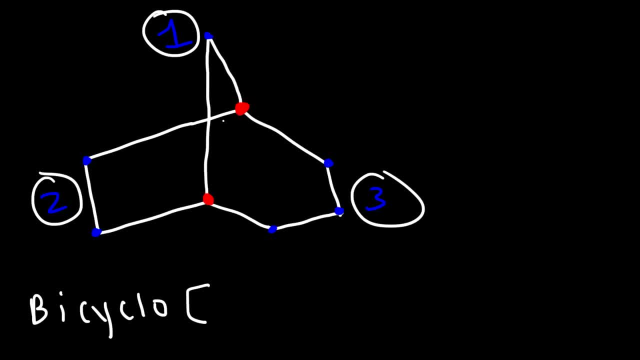 then in the set in order, 3,, 2,, 1.. And then how many carbons do we have in this molecule? It's going to be the sum of these three numbers, 3 plus 2 plus 1, which is 6, plus the two bridgehead carbon atoms. so that's. 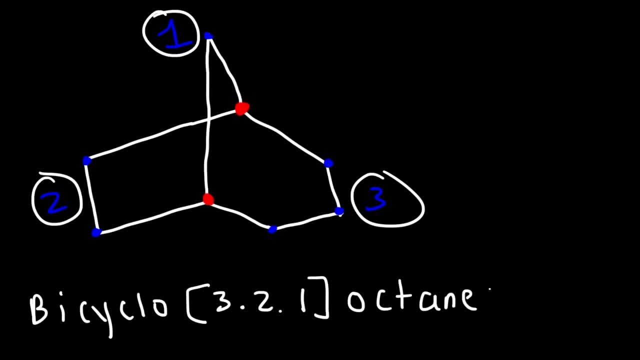 8, so octane. So it's bicyclo 3, 2, 1, octane. To number it, we're going to start with a bridgehead carbon and we need to begin numbering the largest section first. So 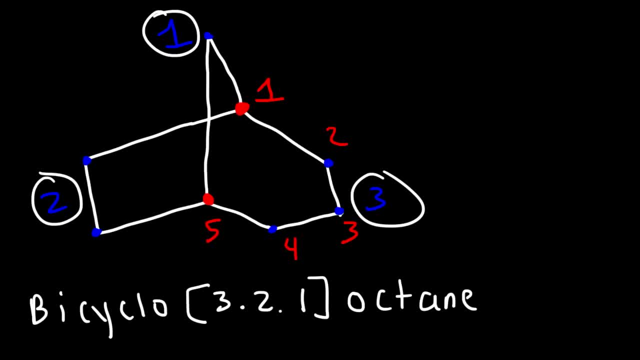 this is going to be 2,, 3,, 4,, 5, and then the smallest section, we're going to count it last- 6,, 7, and then 8, so we have a total of 8 carbons. Go ahead and try these two. 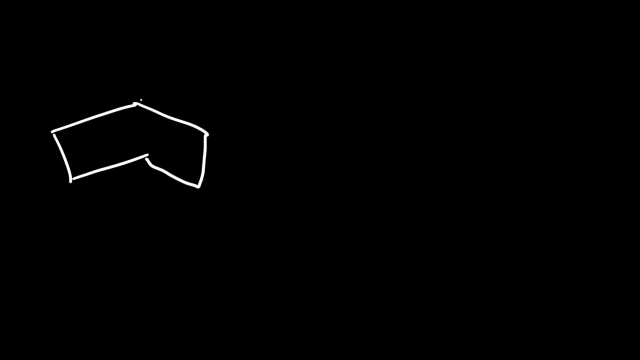 examples and also try this one too. So here are the two bridgehead carbon atoms. We have two carbon atoms on the left side, two on the right side and at the top there's two, So this is going to be called bicyclo, and then 2,, 2,, 2-octane. 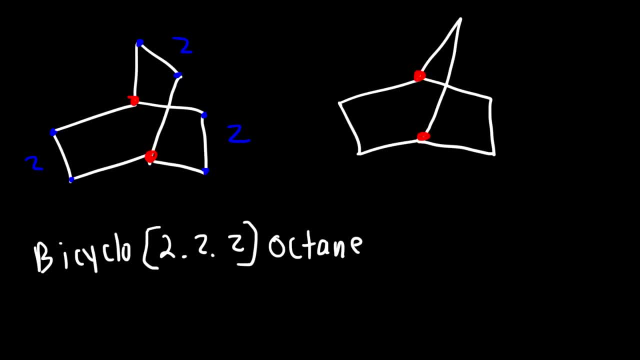 For the structure on the right, here are the two bridgehead carbon atoms. We have two carbon atoms on the left, two on the right and one at the top, so that's going to be called bicyclo 2,, 2, 1, and 2 plus 2 plus 1 is 5, plus the two bridgehead. 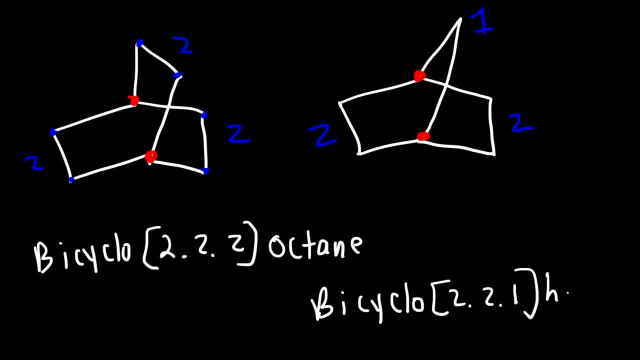 carbon atoms. so that's going to be 7, and so it's going to be heptane. So we can number it this way: Carbon 1, 2, 2-octane. Carbon 1, 2, 2-octane. 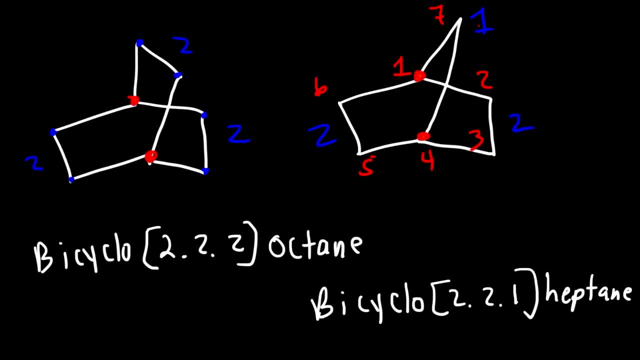 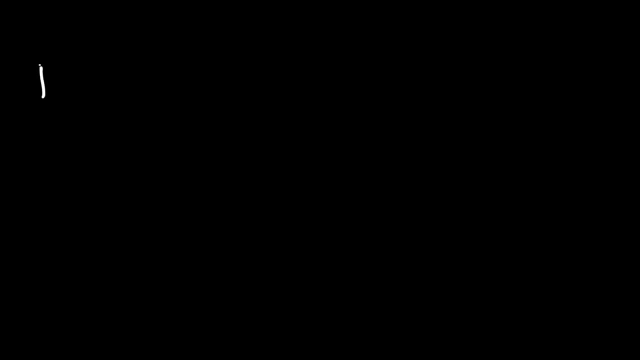 Carbon 1, 2, 2-octane Carbon 1, 2-octane Carbon 1, 2, 2, 2-octane Carbon 1, 2,, 2,, 3,, 4,, 5,, 6, and the last one because it's the shortest link. 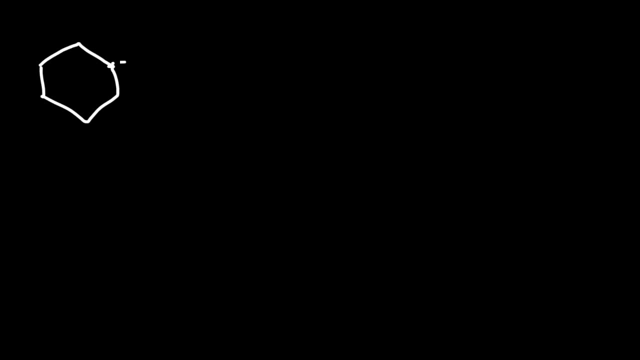 Here are another two examples that you can work on. Try those two. Let's identify the bridgehead carbons, And so we have four carbon atoms on the left side. So what does it do? On the right side there's two carbon atoms and in the middle there's no carbon atoms. 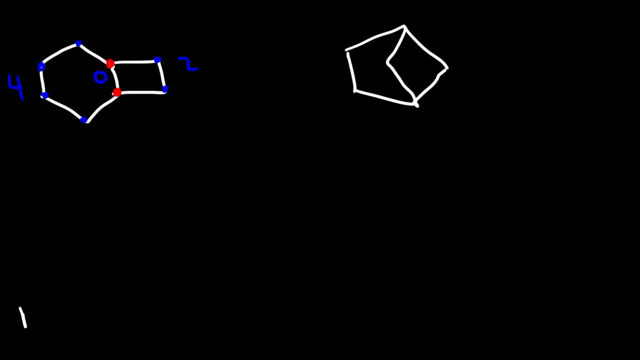 between the two bridgehead carbons, And so this is going to be called bicyclo. in descending order: 4, 2, 0, and we have a total of eight carbon atoms, so octane. So, to number it, we're going to start with the bridgehead carbon and we're going to 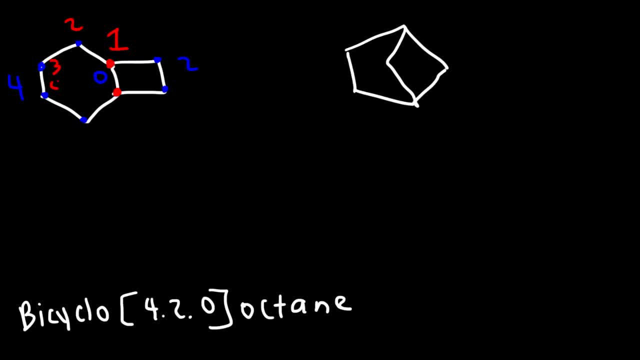 start counting towards the larger ring and then towards the smaller ring. So there's a total of eight carbons in that example. Now for the next one. here are the bridgehead carbons. On this side there's two carbon atoms, in the middle there's one, and on the right 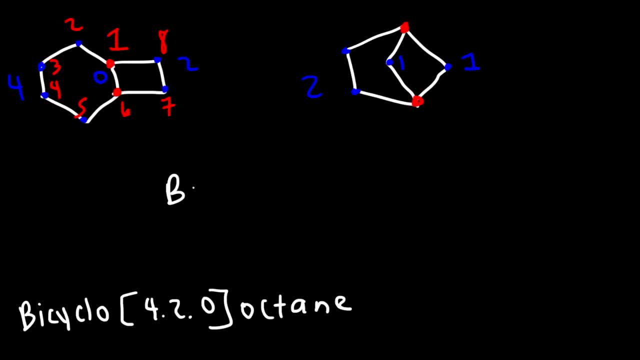 side there's one, So that's going to be called bicyclo, And then, in descending order, 2,, 1, 1, and we have a total of this is four plus the two bridgehead carbons, so six. so that's going to be hexane. 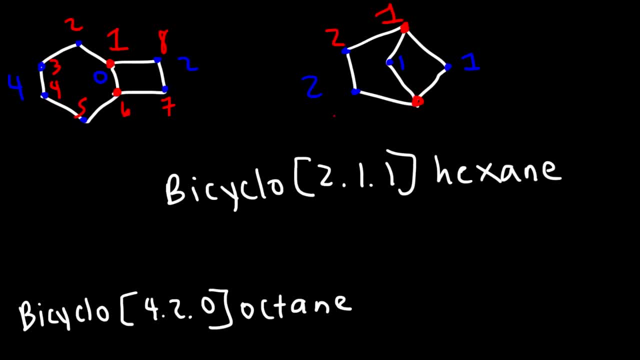 And so to number it, we're going to start with one and then go towards the longest link, and then five, and then the one in the middle will be six. Now let's try one more example, but this time with substituents. 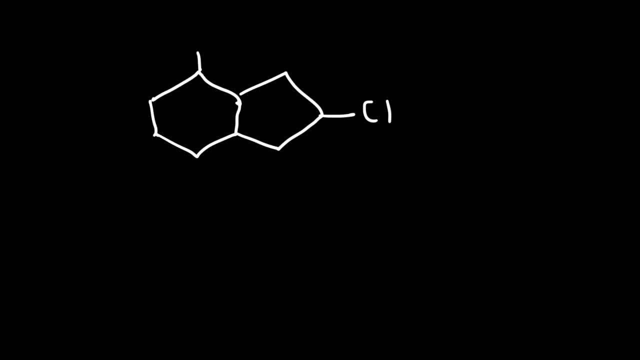 Okay, Feel free to pause the video and try this problem. So let's identify the bridgehead of carbon atoms first, On the left side, there are four carbon atoms, in the middle there's zero, and on the right side we can see that there's three.